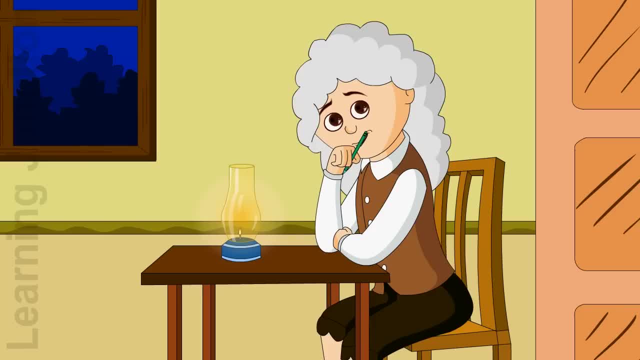 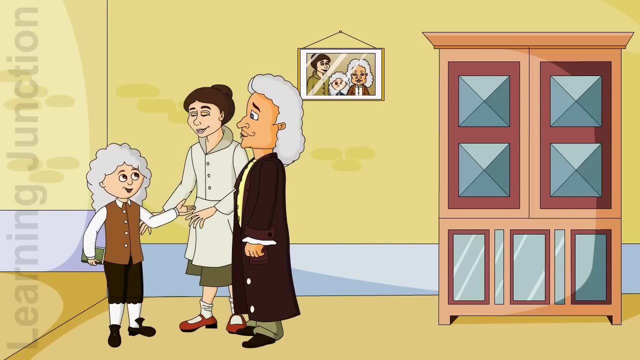 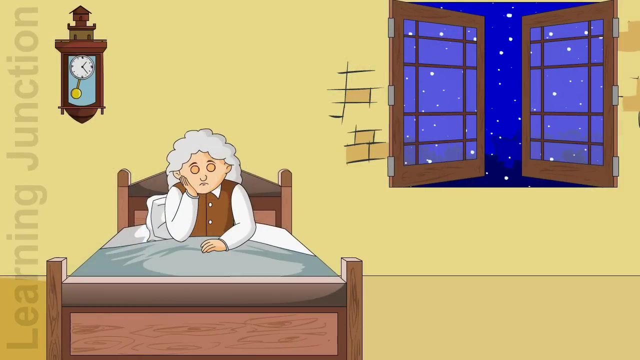 with his friends, but the whole incident made him think as to the apple fell down and not fly up in the air. he asked his parents as to why the apple fell down, but no one could give him a proper answer. this thought bothered him for many, many days. 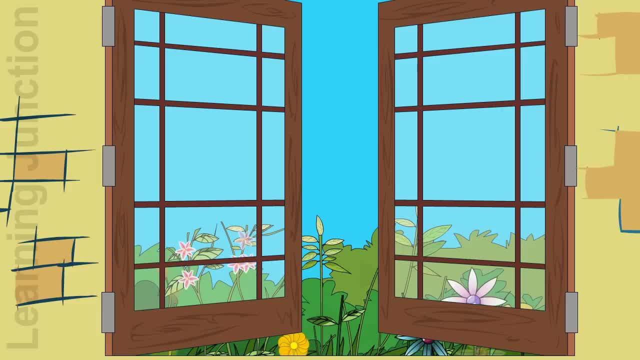 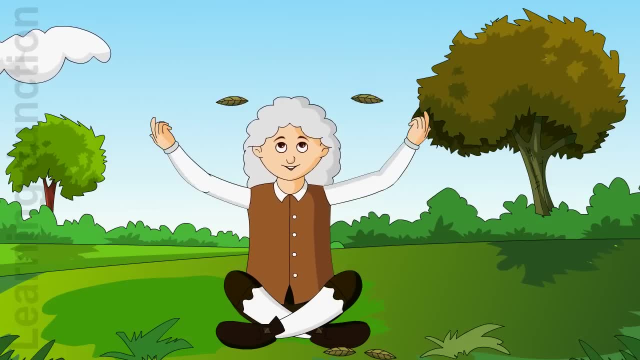 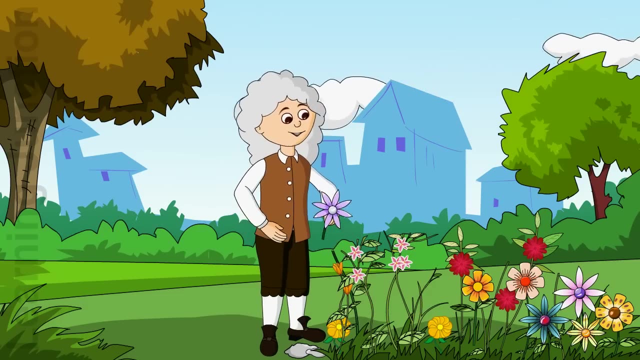 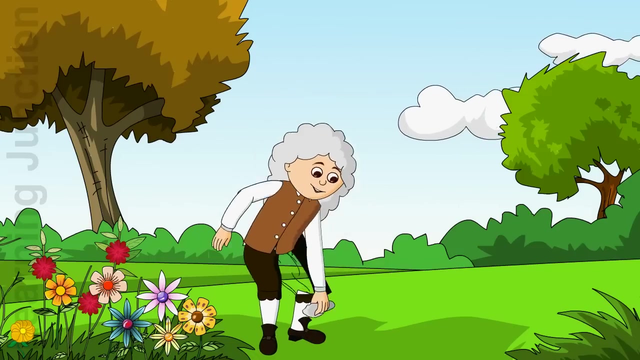 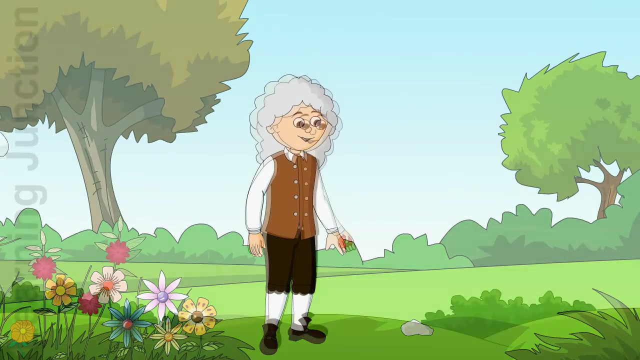 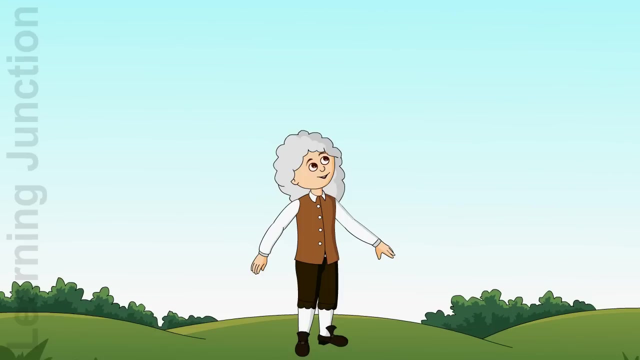 Isaac observed that everything that he would throw in the air would eventually come down. nothing that went up stayed up forever. it would fall down, as if something just pulled it right back to earth. he threw a ball very, very high up in the air, but it also came right back down. he got. 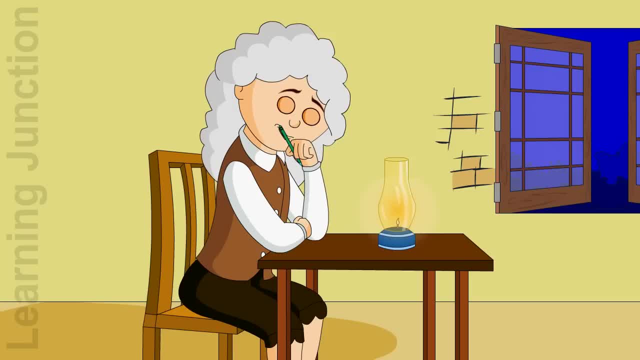 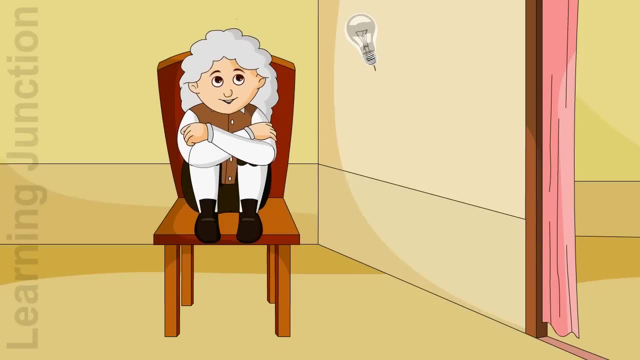 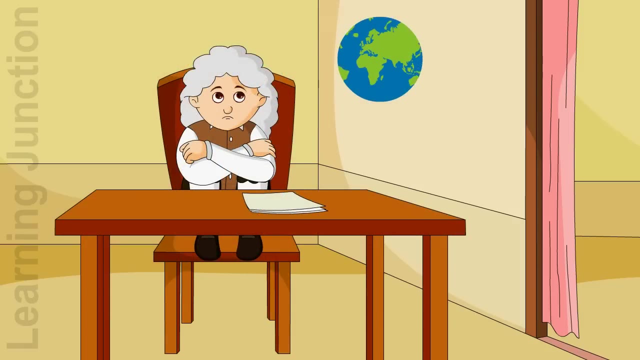 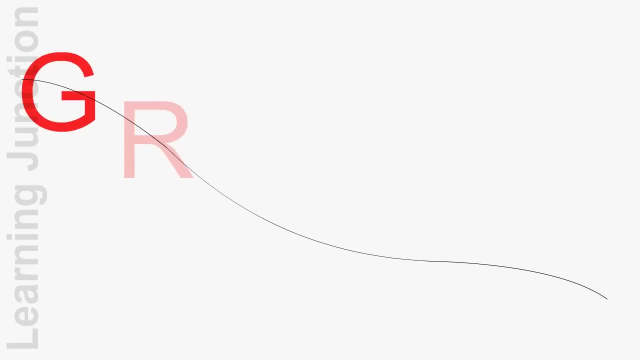 so obsessed with finding an answer that he researched day and night for several years. then he found out that it was earth that would pull everything back down. earth had the power of pulling back, power called gravity. whenever he threw something up in the air, the gravity would pull it right back to earth. gravity was like a string. if something went up, that string called 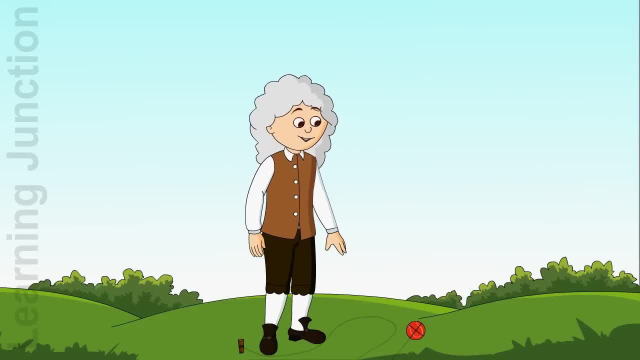 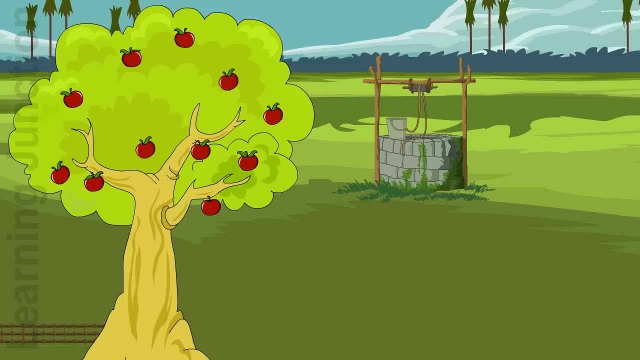 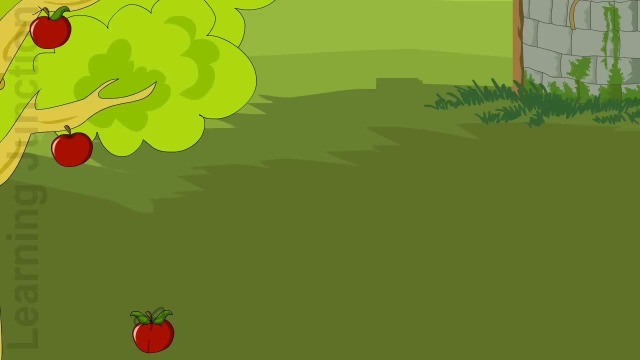 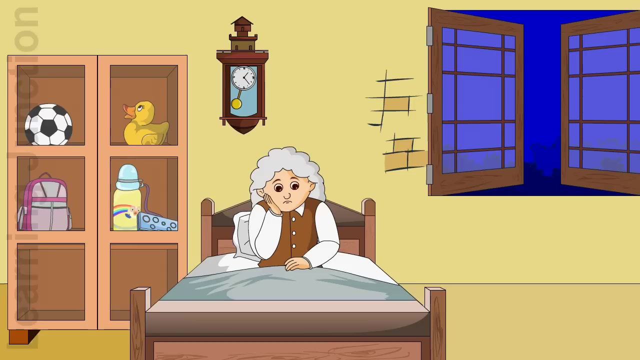 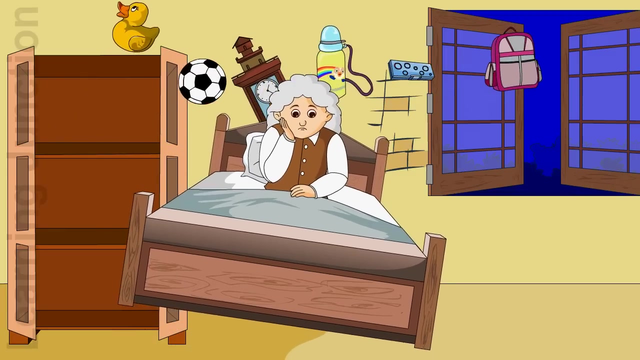 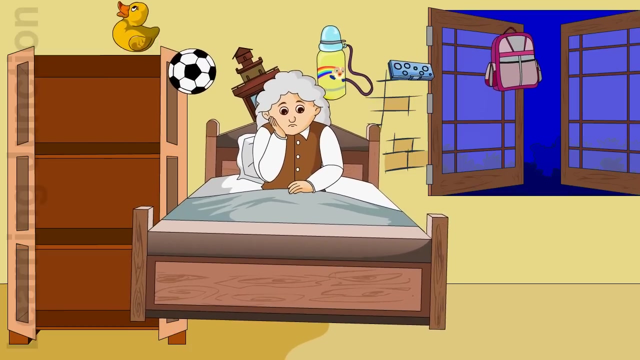 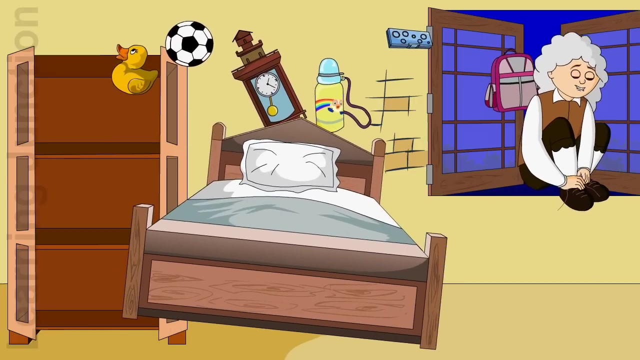 gravity would pull it right back. finally, after years of research, most researchers stopped식. gravity makes sure everything is down on the ground and not flying up in the air. imagine was flying in the air your toys, your bad, your clothes, even you. it would be so hard to play or sleep or get ready for school. Isaac.